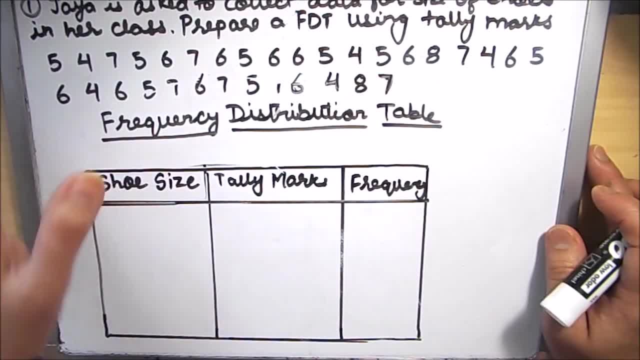 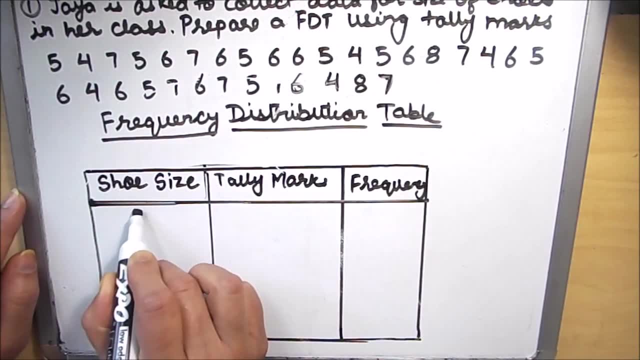 number of shoe sizes we have been given in the, in all the data. So here we see: the lowest or the smallest shoe size is 4, so we will start with 4, the next one is 5, then 6, then 7 and the biggest, 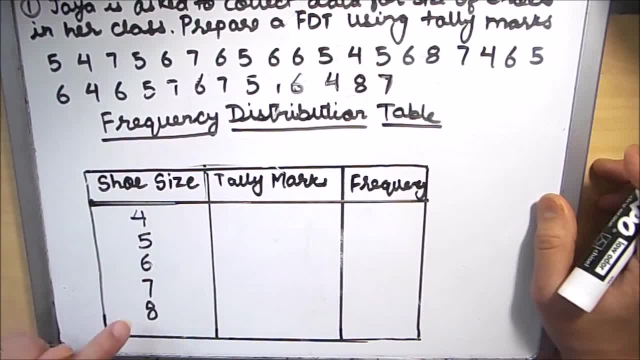 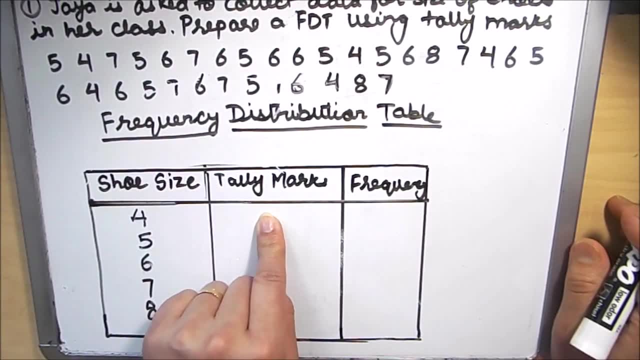 shoe size is 8.. So from 4 to 8 we are going to write the size is the first column. Now the second column is of telemarks. Telemarks tells us which number is appearing how many times here. So we are. 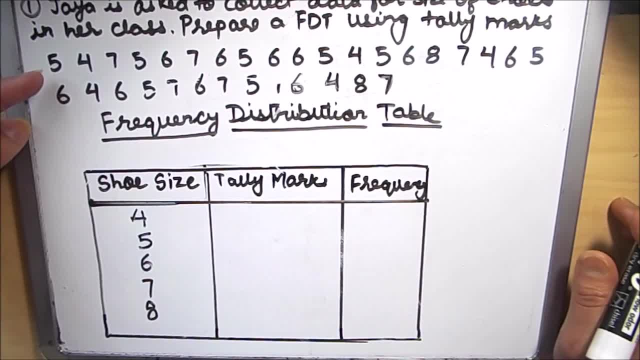 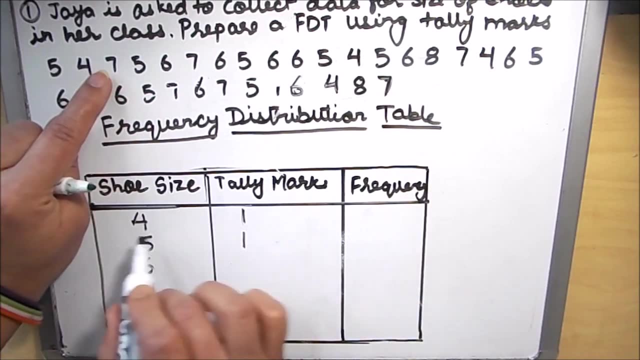 going to start with a data here. The first number or the first shoe size is 5.. So we are going to Now. the next shoe size is 4.. So we are going to mark 1 there in front of the 4.. Next is 7.. 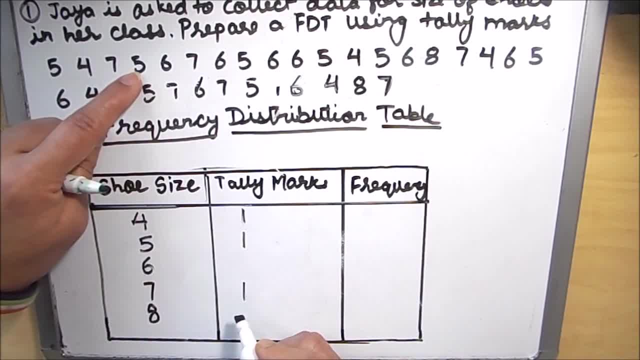 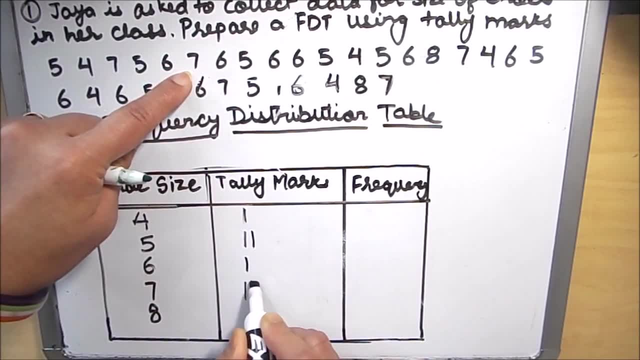 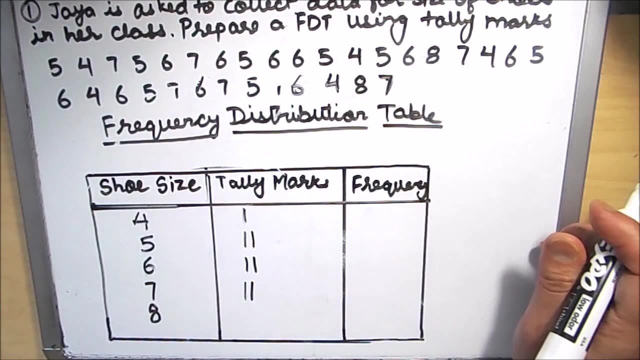 Shoe size: 7. Telemark: 1. Shoe size: 5. Telemark: 2. Shoe size: 6. Telemark: 1. 7,, 2,, 6,, 1, and we go on filling the telemarks according to the numbers given here. Then it's 5., Next is 2.. So we are going to. 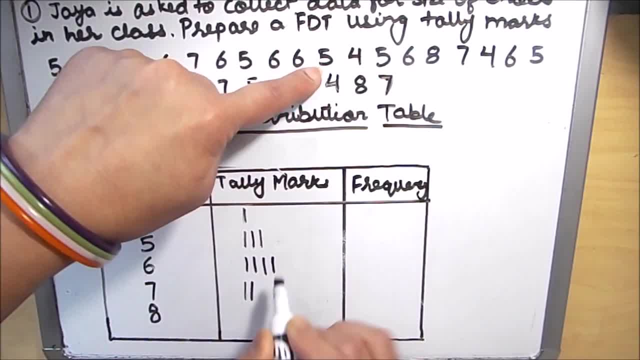 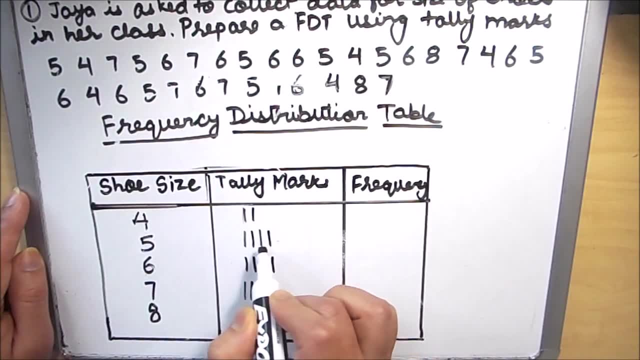 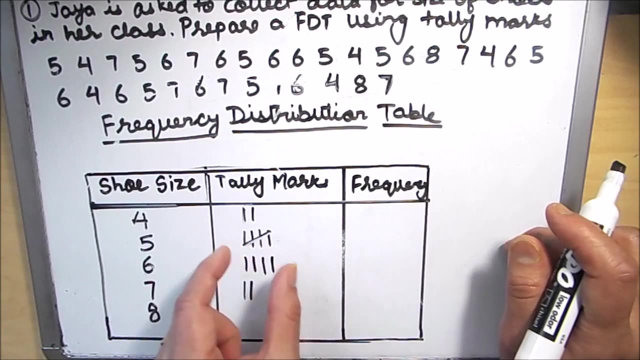 6.. So we will write 1, 1.. Next is 5,, 4,, 5.. So one more 5.. When the number of telemarks is 4, the fifth telemark will come like this: So it is easy to count If we are getting more telemarks. 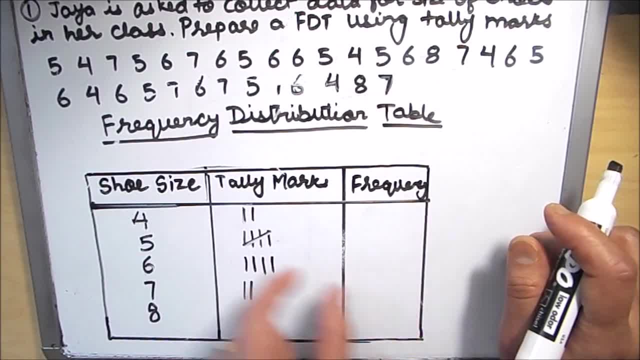 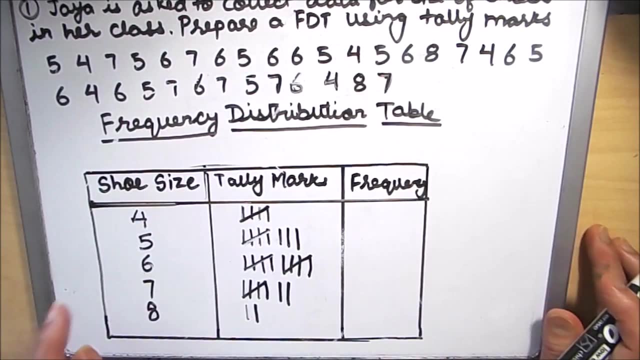 or more bundles like this, so it will be easy for us to count. That's why we make the telemark, fifth telemark as a slanting one, to make a bundle of 5. And then 7.. So we are done with our telemarks Frequency column. we are going to write the 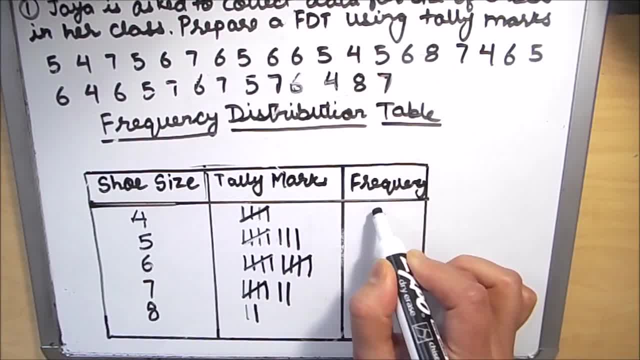 numbers. So here this is a bundle of 5.. So frequency is 5.. Frequency tells us how many people or how many of the same number occurs in the table. So here we can see: the number of people with shoe size 4 is 5.. Shoe size 5,, it is 8..